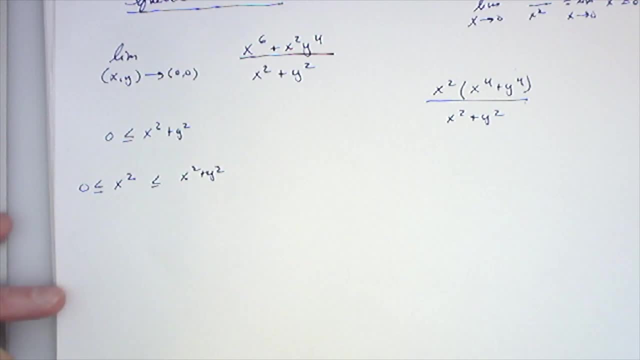 than or equal to x squared plus y squared, And then I can divide everything by x squared plus y squared, so that 0 is less than or equal to x squared over x squared plus y squared, which is less than or equal to 1.. 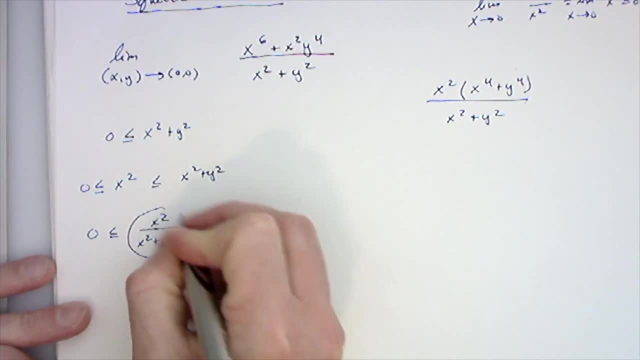 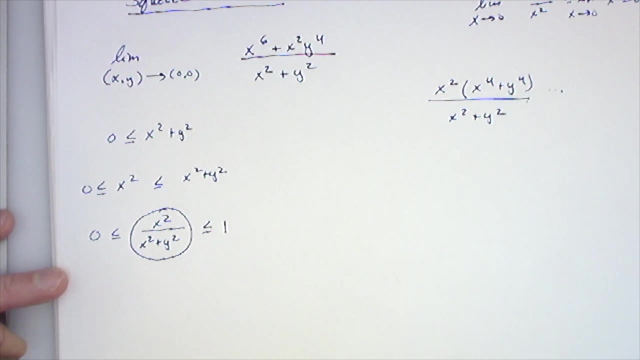 Guettchen, If I divide x squared plus y squared by xj. so this quantity I'm essentially squeezing, except I don't want just that. I really want this thing over here. so I'm going to take this down and multiply it by x to the fourth plus y. 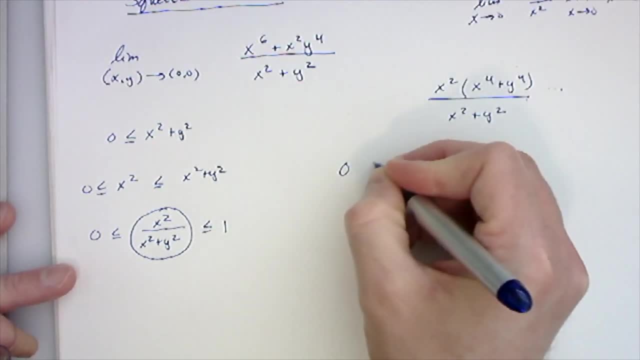 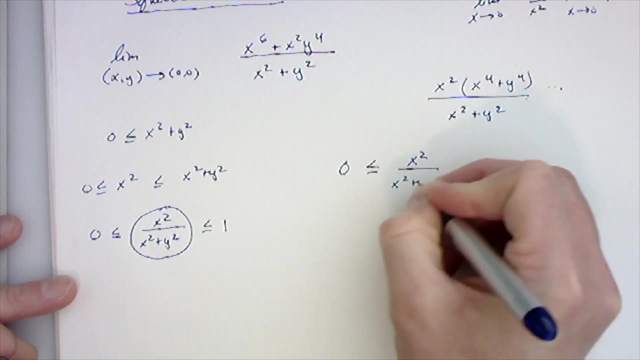 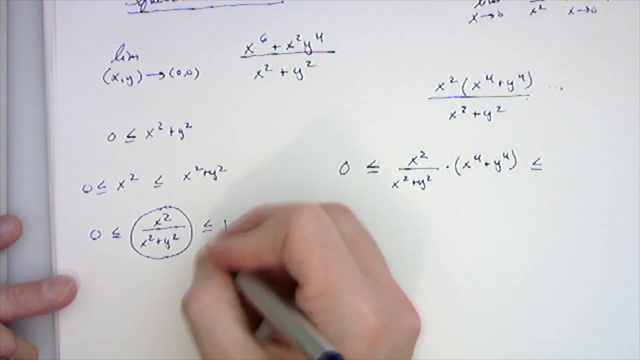 to the fourth, so I'm going to have zero. it's less than or equal to right. so multiplying zero by x to the fourth plus y to the fourth is less than x squared over x squared plus y squared times x to the fourth. plus y to the fourth is less than or equal to one times x to the fourth. 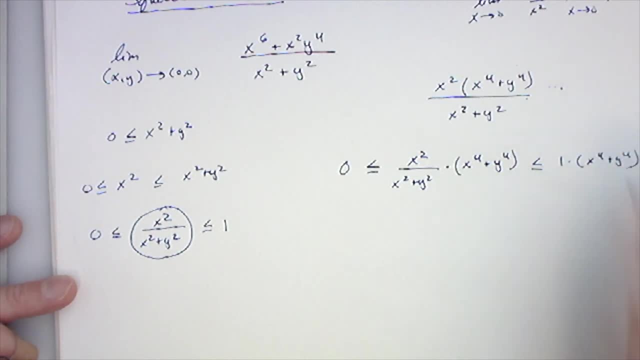 plus y to the fourth. but now I can take the limit of the left side and the right side. so again we the thing we want to find the limit of to be squeezed between two things. the limit as xy goes to zero. zero of zero is obviously zero. the limit is x, y, whoops, I just 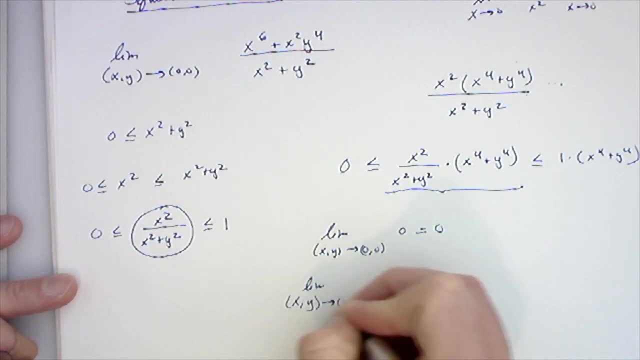 pushed a button. hopefully didn't affect anything goes to zero. zero of x to the fourth plus y to the fourth. I can just plug in zeros and get zero and since then x, nothing, and so I can just plug in zero, zero of x to the fourth. so I can just plug in zero and get zero and since then I can just closes. 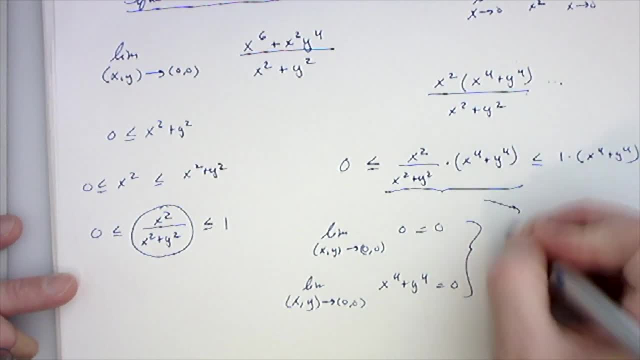 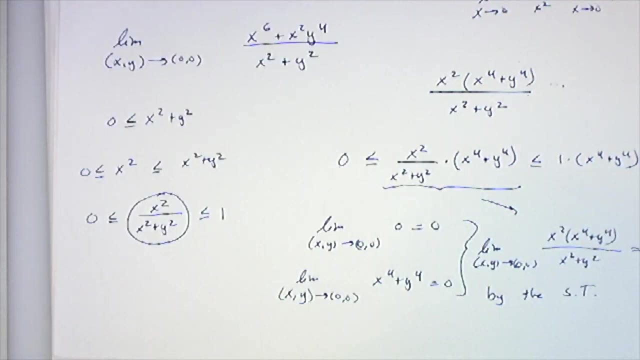 is zero and this is zero. it means that the middle thing limit is x. y goes to zero. zero of x squared times- x to the fourth plus y to the fourth- over x squared plus y squared, must equal zero by the squeeze term. so i hope that kind of helps clarify what you're looking for. you're usually looking for. 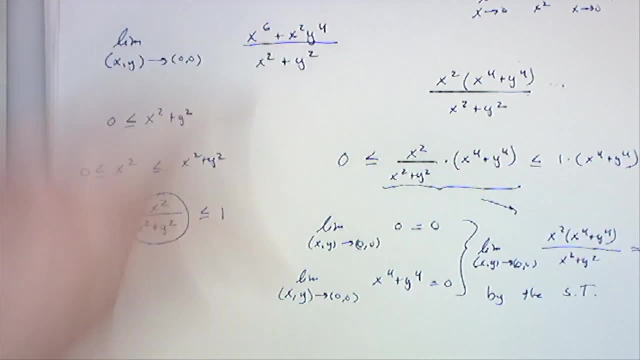 something to be less than one, so you can say that, then the inside part, so i got this little something. i could multiply that by that. say that this inside part ends up being less than something that you can actually take the limit of and bigger than usually- zero, okay.